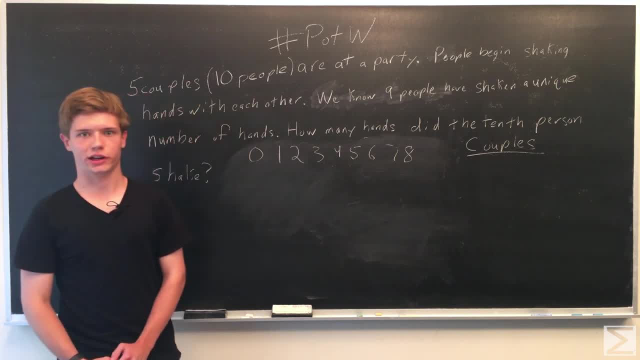 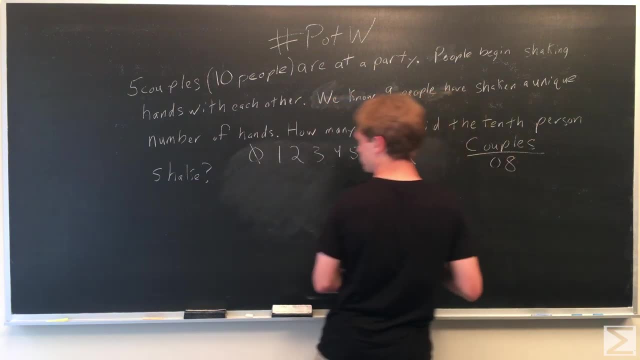 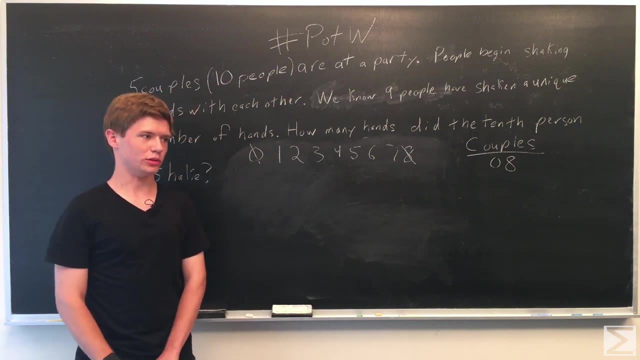 so would thus not be shaking hands with her partner. So we can eliminate them immediately. So now we're left with a group of eight people. They're labeled one through seven and then the mysterious tenth person, And because we know that they've all shaken hands within this group, 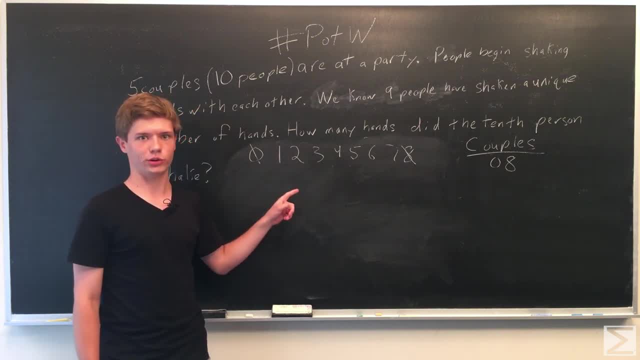 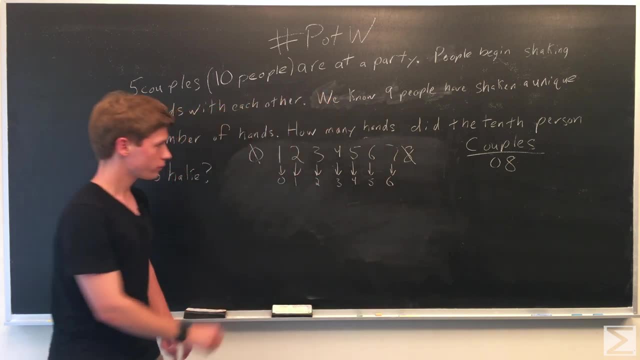 or they've all shaken hands with eight. we can subtract one from each of their totals and get a new subgroup. So now we have a similar situation, but just with a slightly smaller big number. And so now we know out of this subgroup, six has shaken hands with one person. 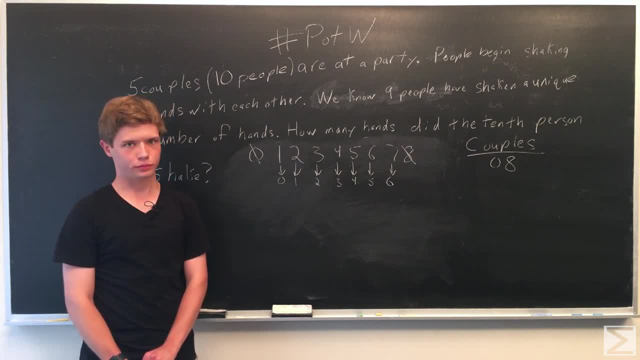 and so now we know out of this subgroup six has shaken hands with everyone except his partner and himself. So that would mean that his partner would also be- or his partner would be- zero. so we know they're a couple. So in the couples list we can cross off one and seven. 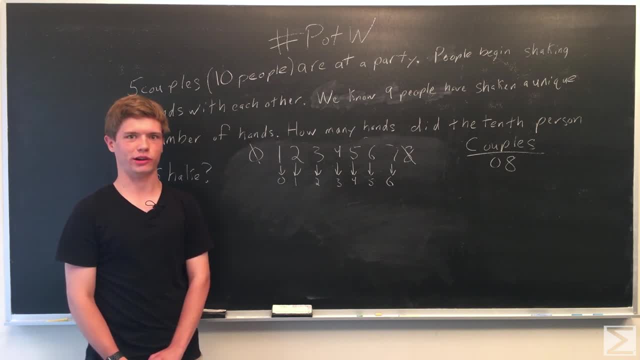 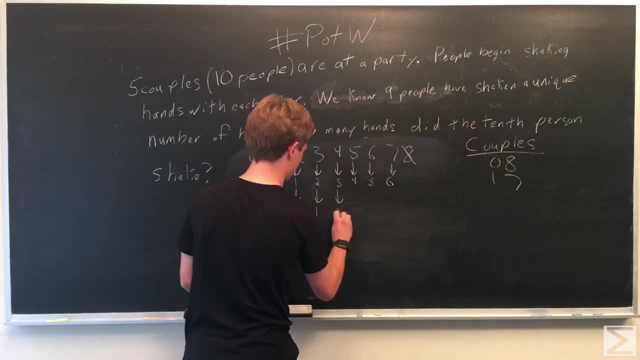 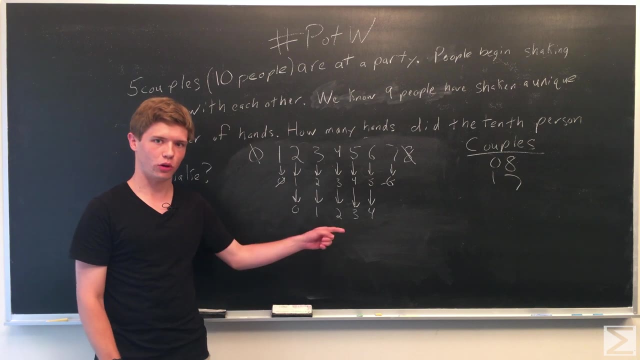 And now we do the same thing that we did in the previous step: We're going to subtract one from everyone's total and have a smaller subgroup to work with. So again in this subgroup, the person labeled four will have shaken hands with everyone in the group. 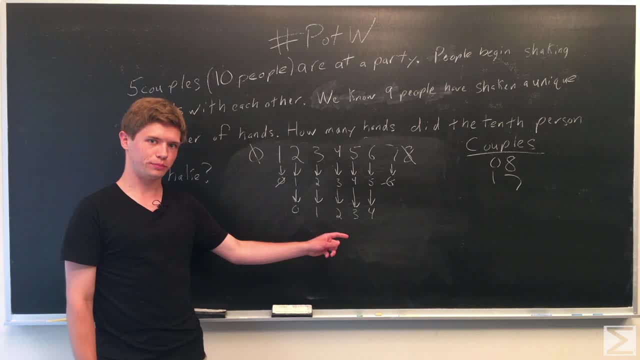 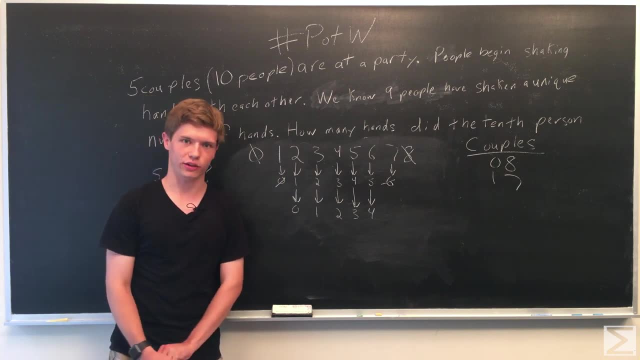 and the person labeled zero will have shaken hands with no one in the group. So we eliminate them, subtract one from the remaining total and then do it again. So now we're down to the final four people. We are left with the mysterious person, the mysterious person's partner. 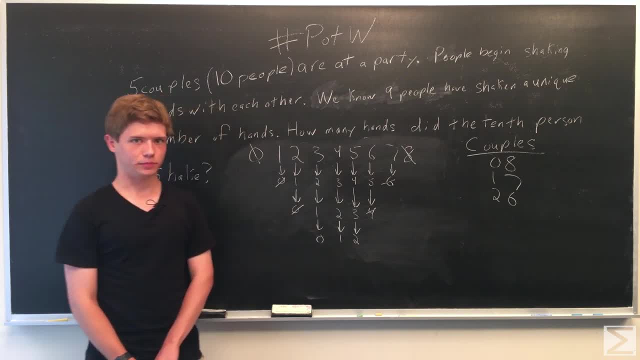 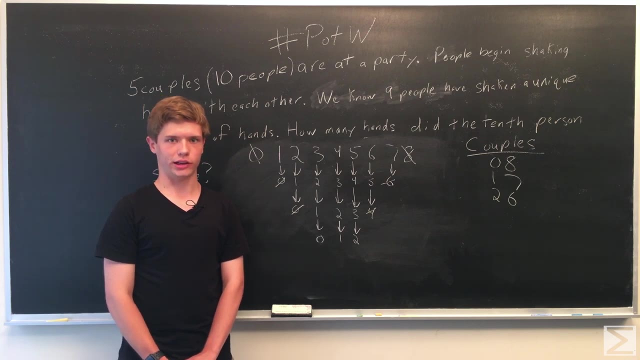 and one other couple, and we know that the person labeled two has shaken hands with the mysterious person and their partner and has not shaken hands with their own partner, who's labeled zero, So we can assume that they are a couple as well. we can eliminate them. 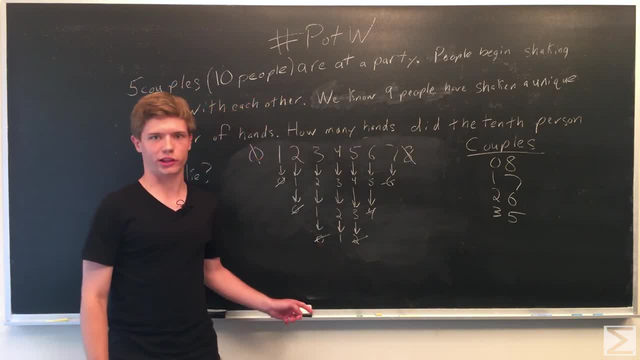 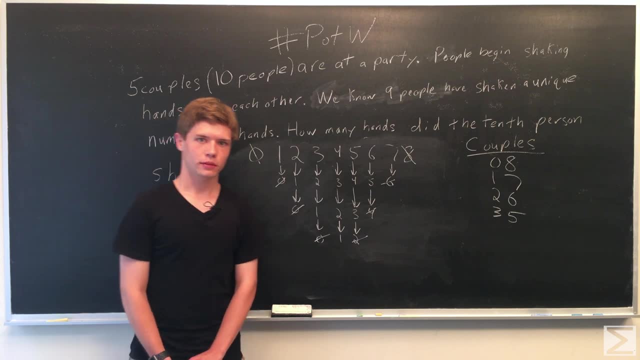 number one. So now we're left with someone who, if we subtract one like the previous steps, will be left with zero. So this person will end up being the mysterious person's partner. And now we look at the previous steps and figure out how many times the mysterious person has had their hand shaken.